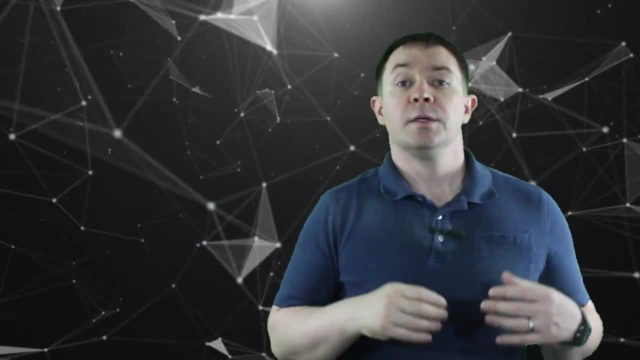 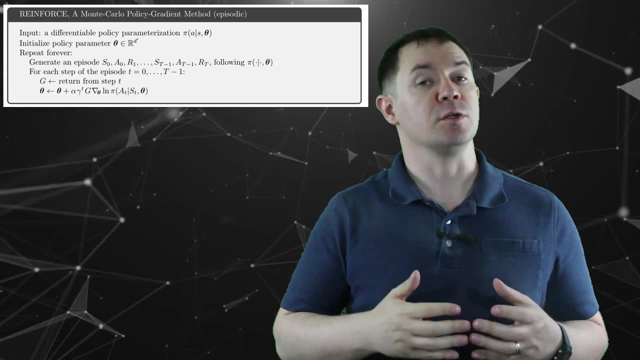 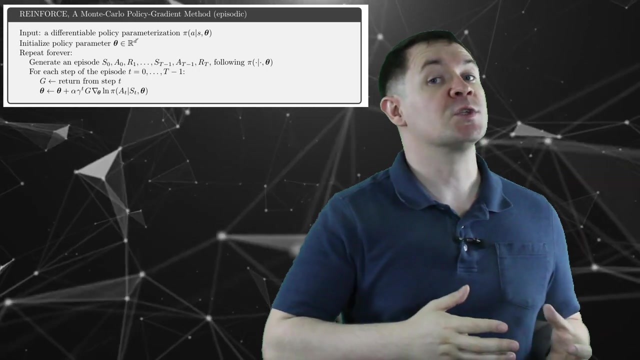 do it, Let's get to it. So here's a basic idea behind policy gradient methods. A policy is just the probability distribution the agent uses to pick actions. So we use a deep neural network to approximate the agent's policy. The network takes observations of the environment as input. 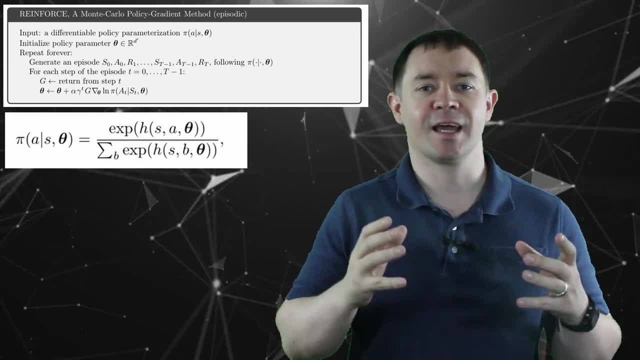 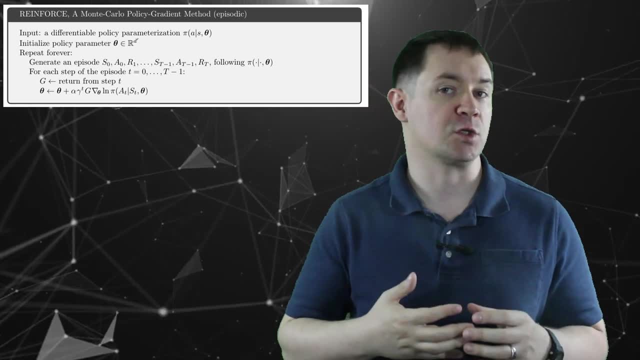 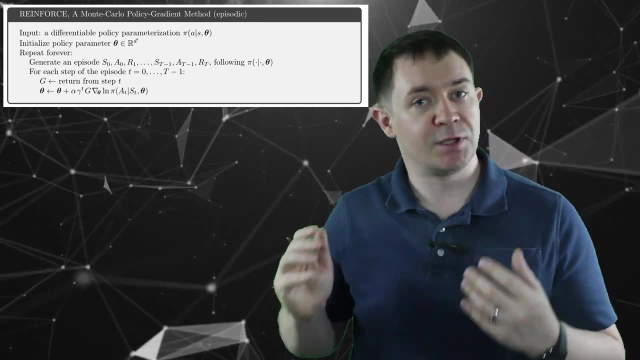 and outputs actions selected according to a softmax activation function. Next, generate an episode and keep track of the states, actions and rewards in the agent's memory. At the end of each episode, go back through these states actions and rewards and compute the discounted future. 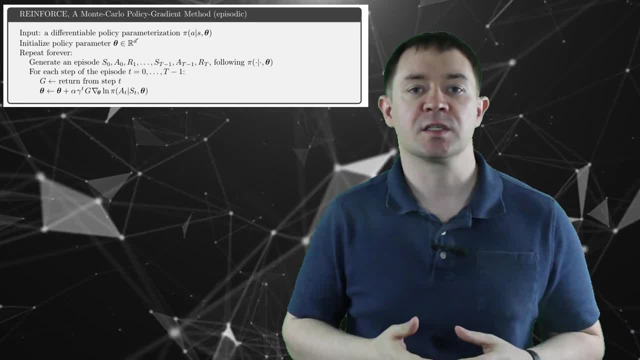 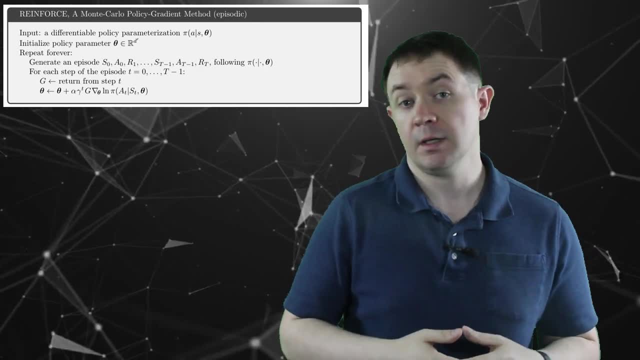 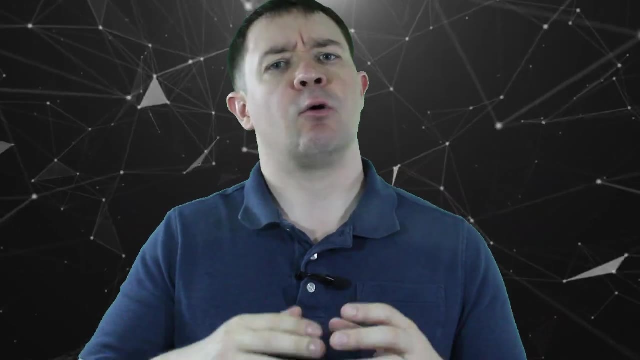 returns. Use those returns as weights and the actions the agent took as labels to perform backpropagation and update the weights of your deep neural network. Then just repeat until you have a kick-ass agent. Simple, yeah, So now we know the what. let's unpack how all this works and why. 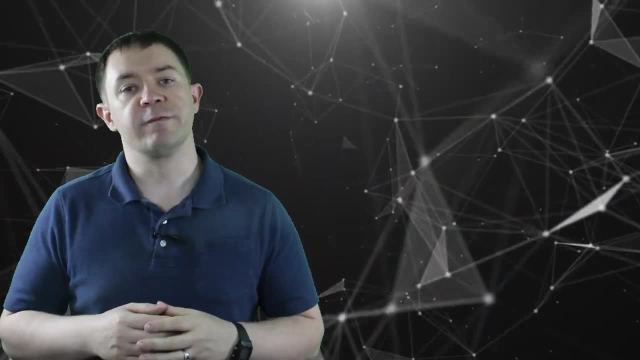 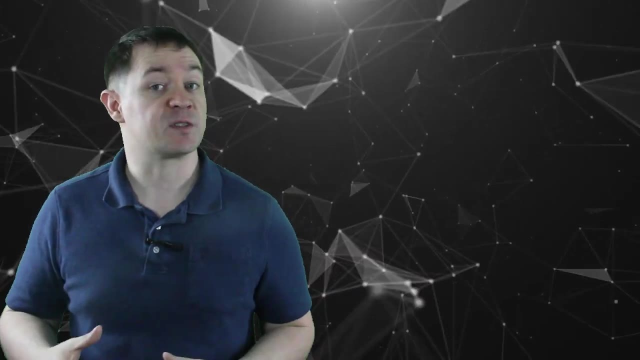 it's something worth doing. Remember, with reinforcement learning we're trying to maximize the agent's performance over time. Let's say the agent's performance is characterized by some function, j, And it's a function of the weights theta of the deep neural network. So our update rule for theta: 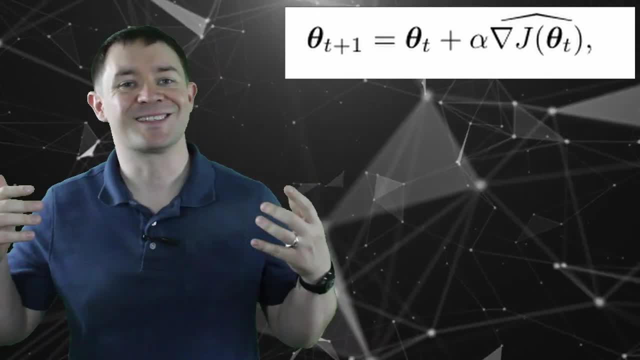 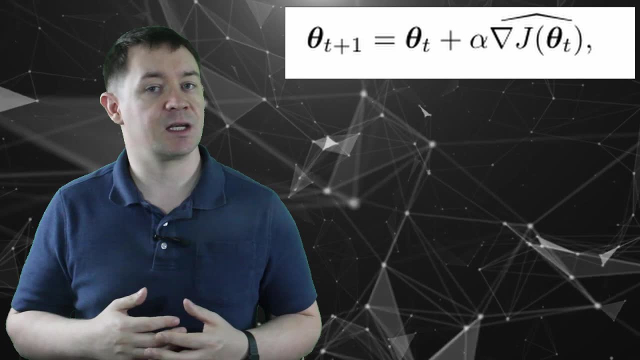 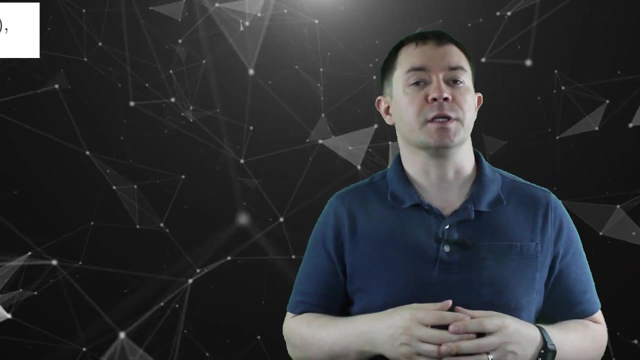 is that the new theta equals the old theta plus some learning rate times the gradient of that performance metric. Note that we want to increase performance over time, So this is technically gradient ascent instead of gradient descent. The gradient of this performance metric is going to be proportional to some overstates, for the amount of time we spend in any given state. 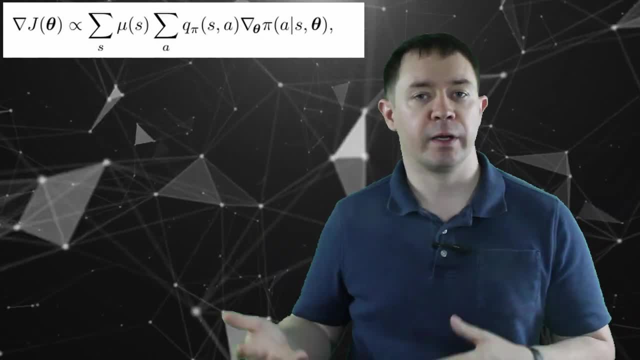 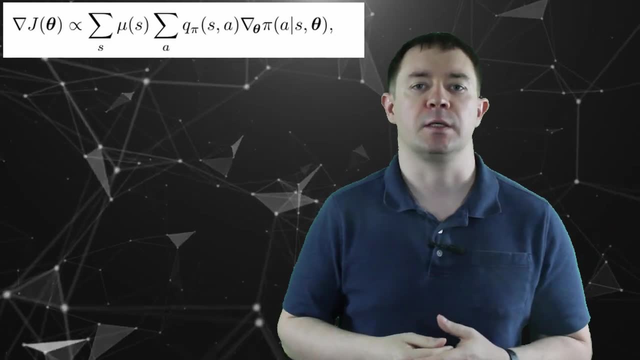 and a sum over actions for the value of the state, action pairs and the gradient of the policy, where, of course, the policy is just the probability of taking each action. given we're in some state, This is really an expectation value and, after a little manipulation, 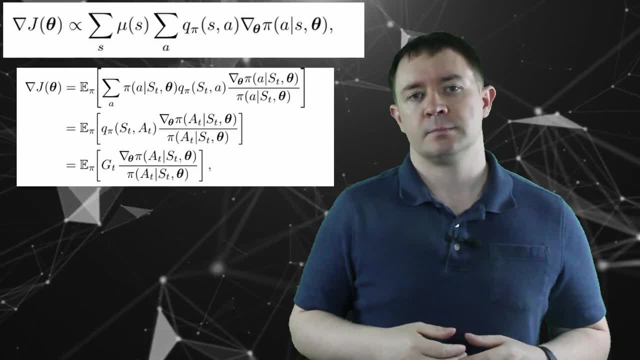 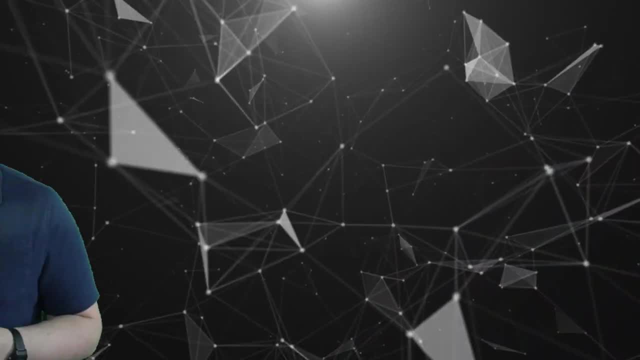 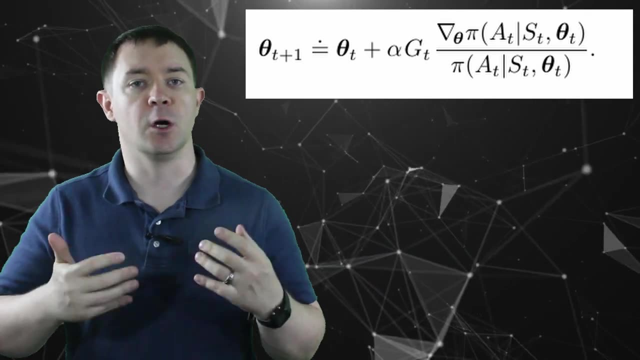 we arrive at the following expression: When you plug that into the update rule for theta, you get this other expression. There are two important features here. This g sub t term is the discounted future returns we referenced in the opening, and this gradient of the policy divided by the policy is a vector. 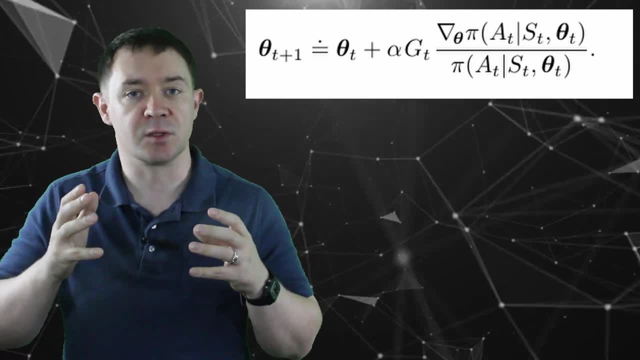 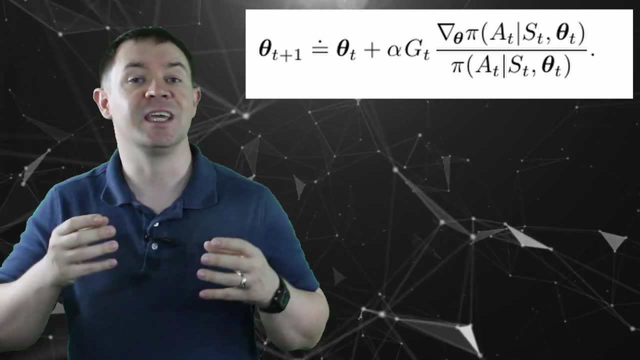 that tells us the direction and policy space that maximize the chance that we repeat the action. a, sub t. When you multiply the two, you get a vector that increases the probability of taking actions with high expected future returns. This is precisely how the agent learns over time. 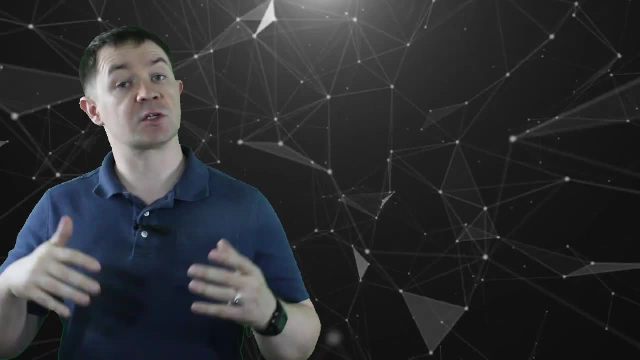 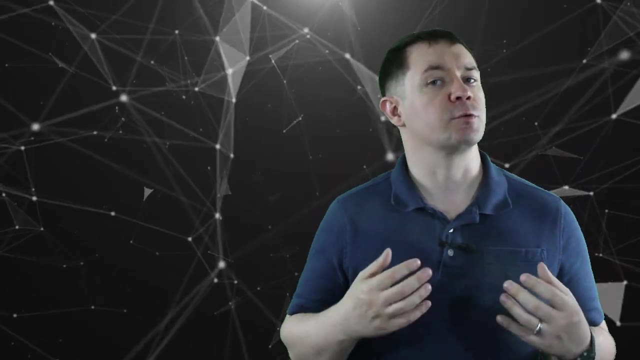 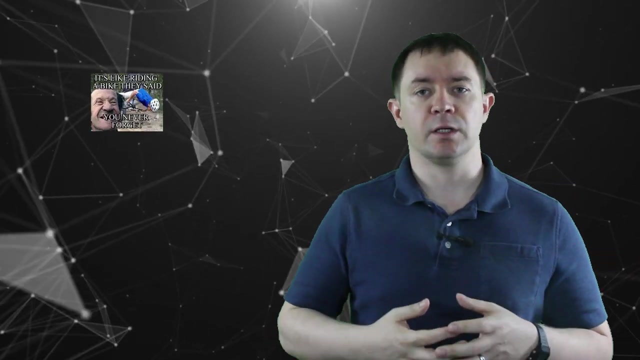 and what makes policy gradient methods so powerful. This is called the reinforce algorithm, by the way. If we think about this long enough, some problems start to appear. For one, it doesn't seem very sample efficient. At the top of each episode we reset the agent's memory, so it 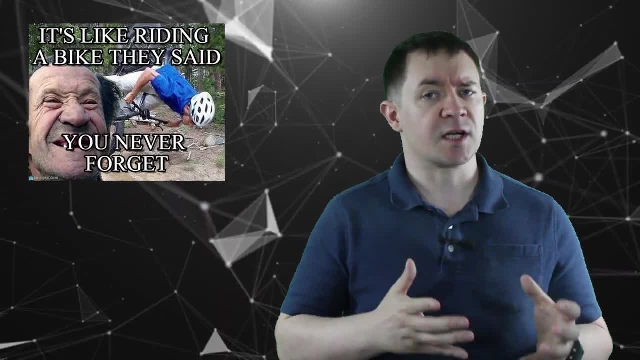 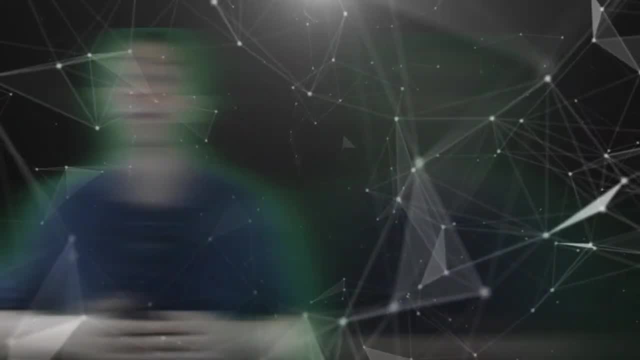 effectively discards all its previous experience. Aside from the new weights that parameterize its policy, it's kind of starting from scratch. after every time it learns Worse. yet if the agent has some big probability of selecting any action in any given state, how can we control the 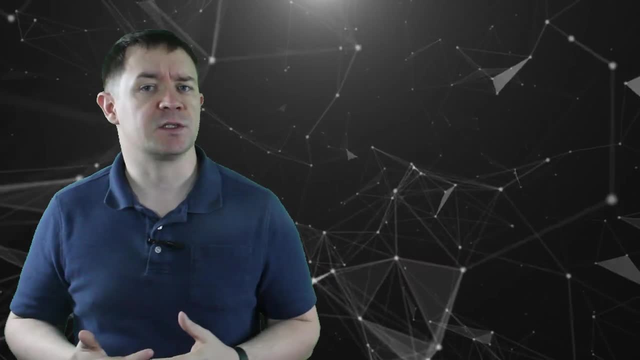 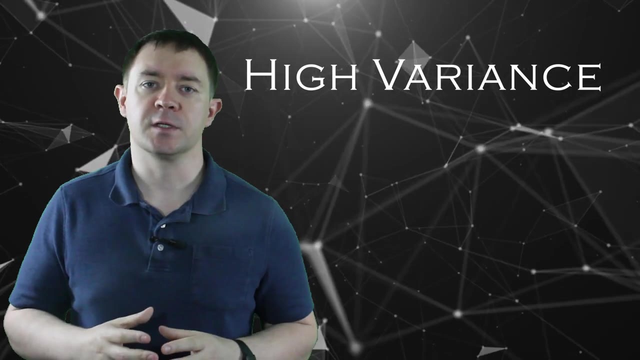 variation between the episodes. For large state spaces, aren't there way too many combinations to consider? Well, that's actually a non-trivial problem with policy gradient methods and part of the reason our agent wasn't so great at Space Invaders. Obviously, no reinforcement learning. 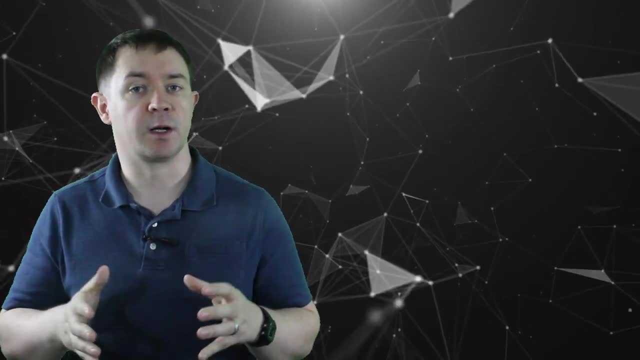 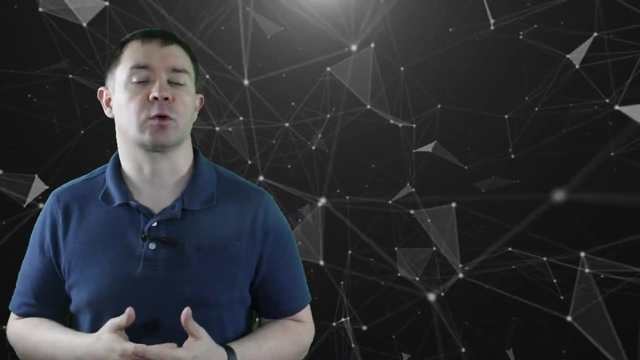 method is going to be perfect and we'll get to the solution to both of these problems here in a minute. But first let's talk about why we would want to use the reinforcement learning method. The policy gradient method is a pretty different approach to reinforcement learning. Many 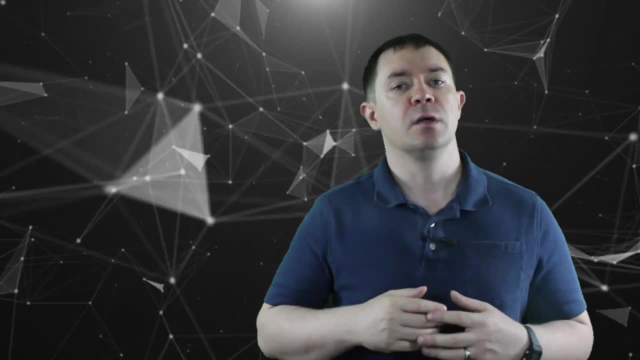 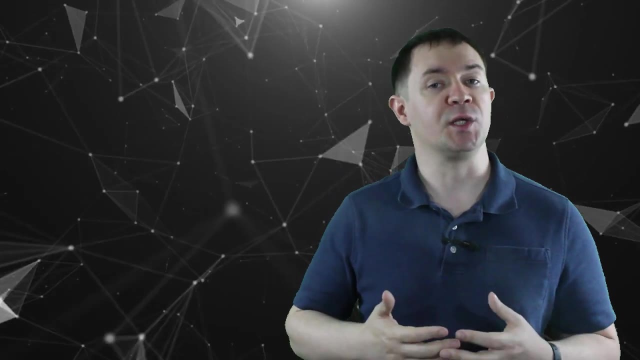 reinforcement. learning. algorithms like deep Q learning, for instance, rely on estimating the value of a state or state-action pair. In other words, the agent wants to know how valuable each state is, so that its epsilon gradient policy can let it select the action that leads to the most. 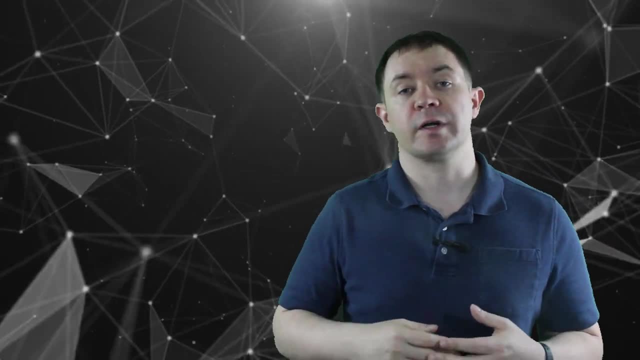 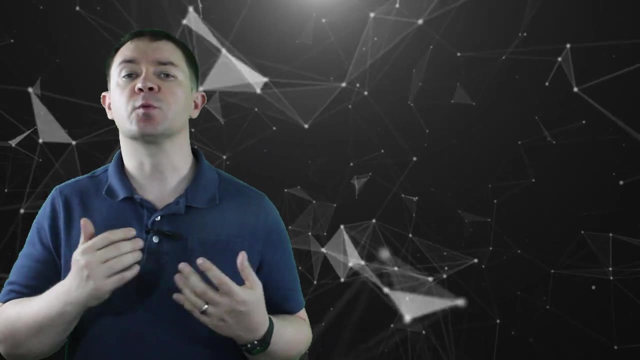 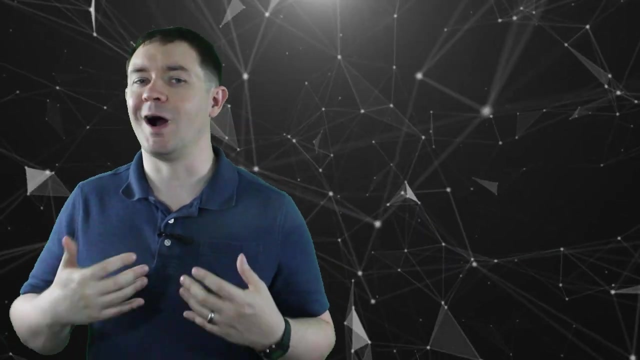 valuable states. The agent repeats this process over and over, occasionally choosing random actions to see if it's missing something. The intuition behind epsilon-greedy action selection is really straightforward: Figure out what the best action is and take it. Sometimes do other stuff to make sure you're not wildly wrong. Okay, that makes sense, but this assumes. 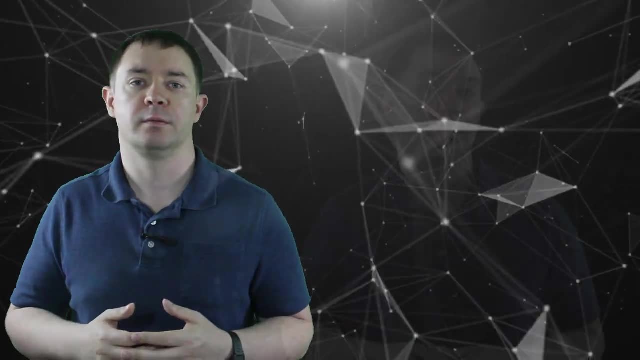 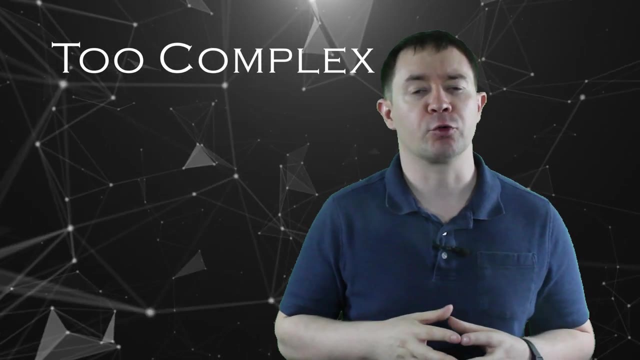 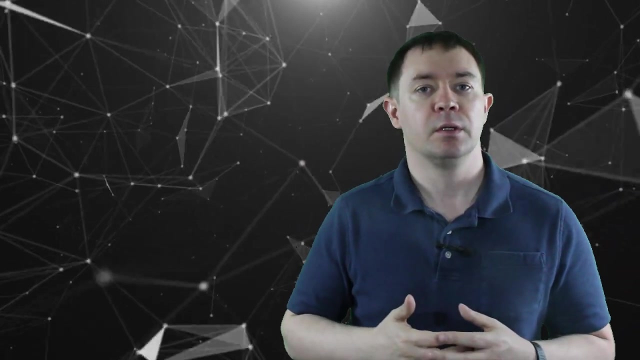 that you can accurately learn the action value function to begin with. In many cases, the value or action value function is incredibly complex and really difficult to learn on realistic timescales. In some cases, the optimal policy itself may be much simpler and therefore easier to. 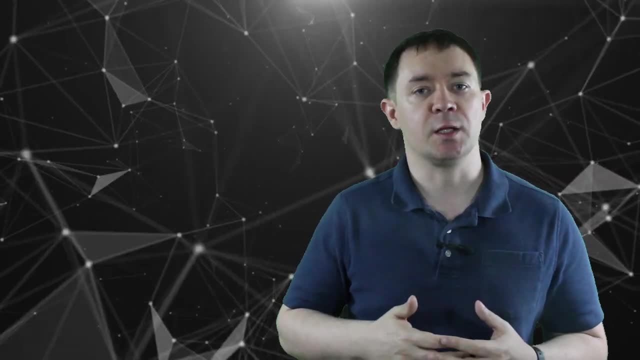 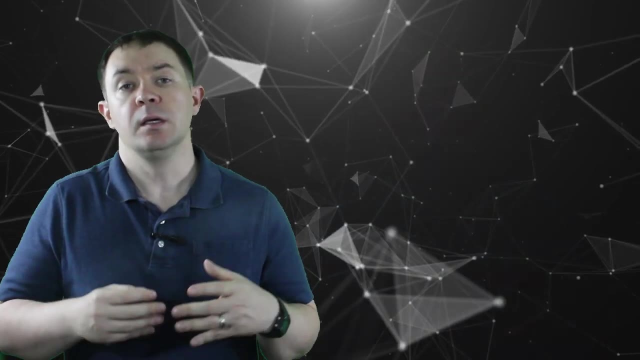 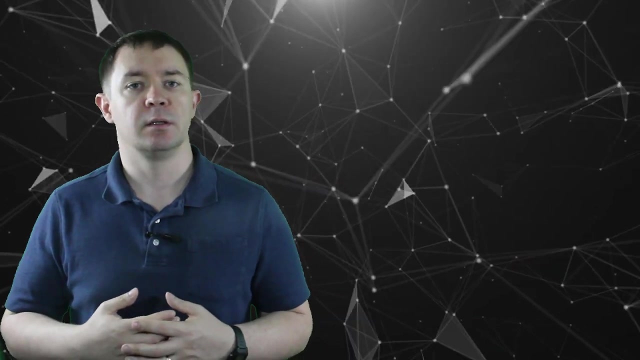 approximate. This means the policy gradient agent can learn to beat certain environments much more quickly than if it relied on an algorithm like deep Q learning. Another thing that makes policy gradient methods attractive is what if the optimal policy is actually deterministic In really simple environments? 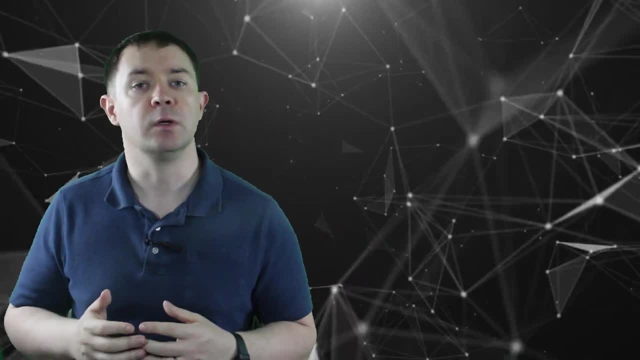 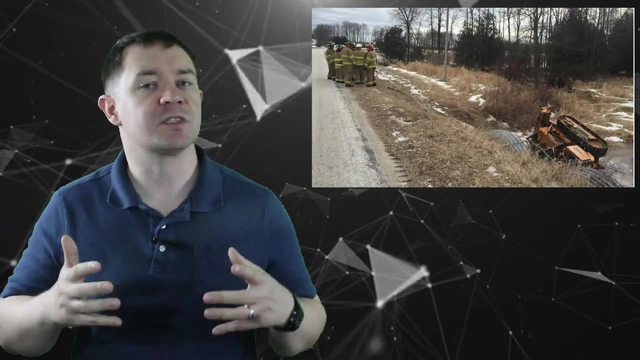 with an obvious deterministic policy, like our grid world example. keeping a finite epsilon means that you keep on exploring even after you've found the best possible solution. Obviously, this is suboptimal. For more complex environments, the optimal policy may very well. 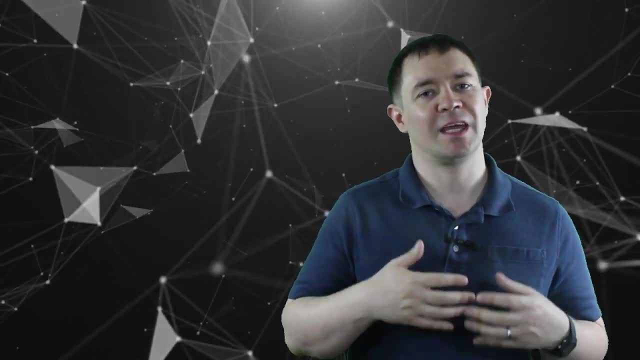 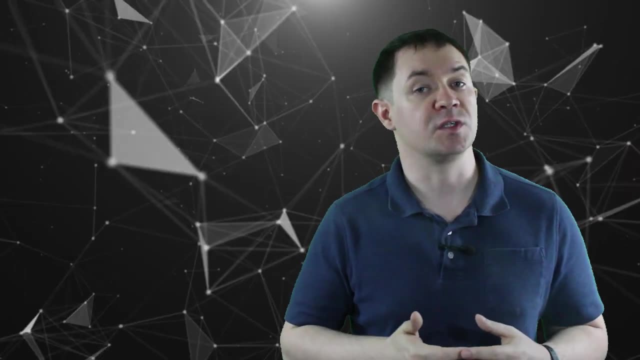 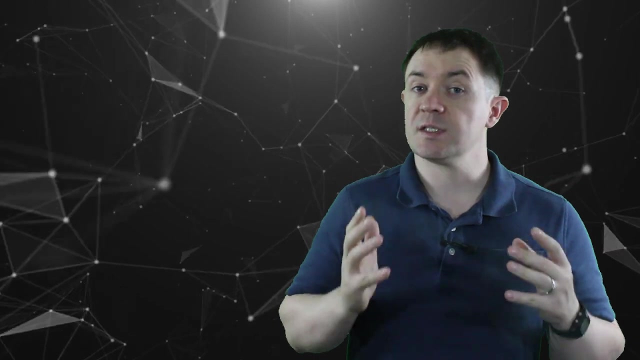 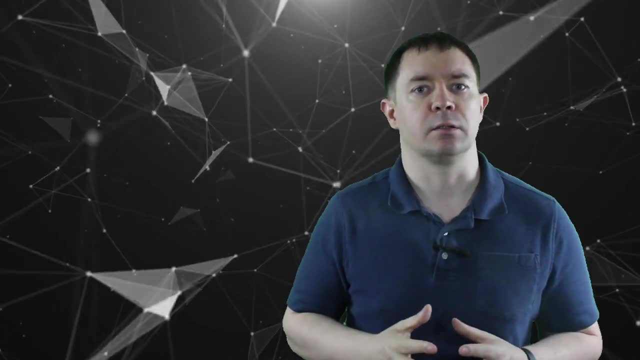 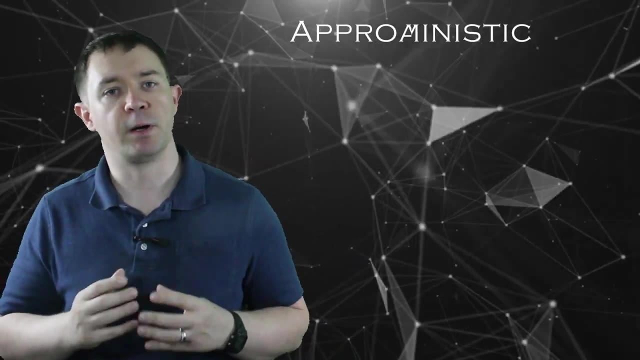 true for all the other models of learning, but it's not always the case. This is certainly true, but how can we know how quickly to decrease epsilon? The beauty of policy gradients is that, even though they are stochastic, they can approach a deterministic policy. over time, Actions that are optimal will be selected. 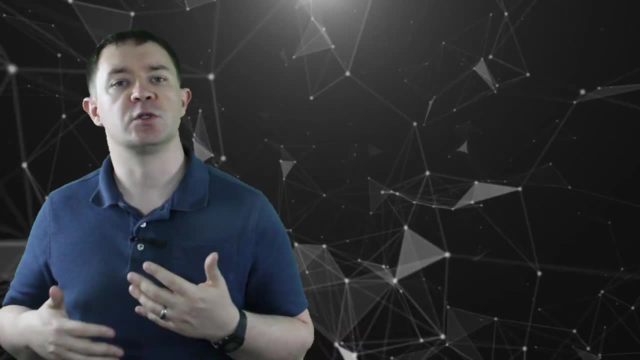 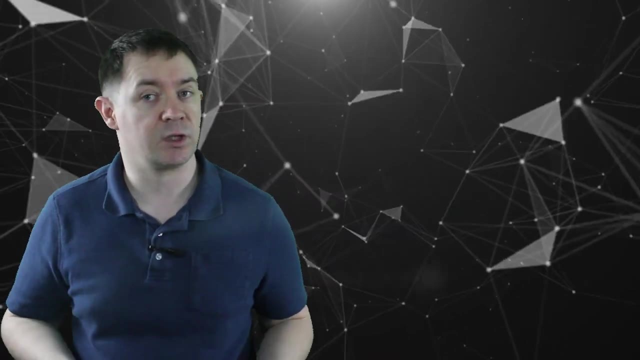 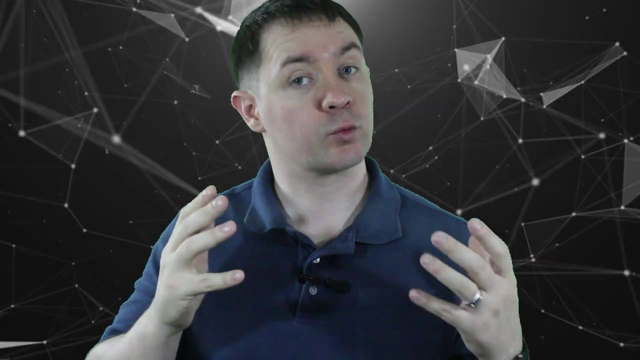 more frequently, and this will create a sort of momentum that drives the agent towards that optimal deterministic policy. This really isn't feasible in action value algorithms that rely on epsilon, greedy or its variations. So what about its shortcomings? As we said earlier, there are really big variations between episodes, since each time the agent visits, 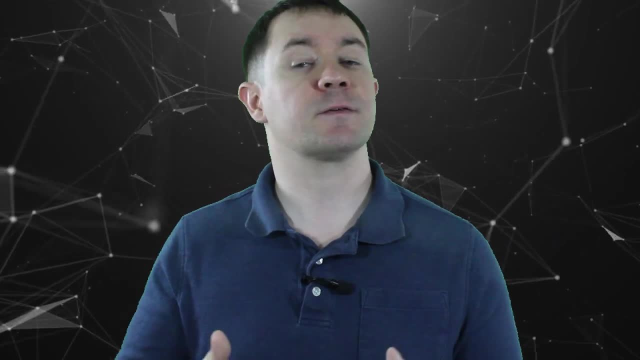 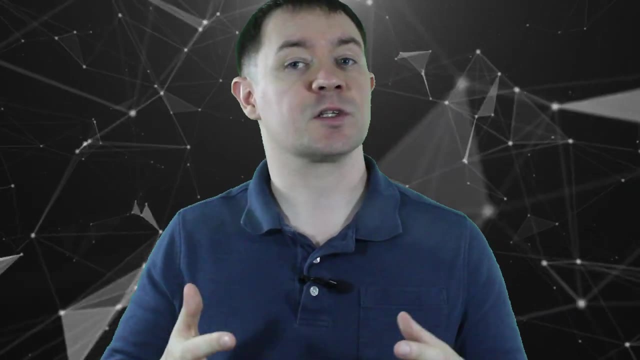 a state, it can choose a different action, which leads to radically different future returns. The agent also doesn't make very good use of its prior experience, since it discards them after each time it learns. While they seem like showstoppers, they have some pretty straightforward solutions.